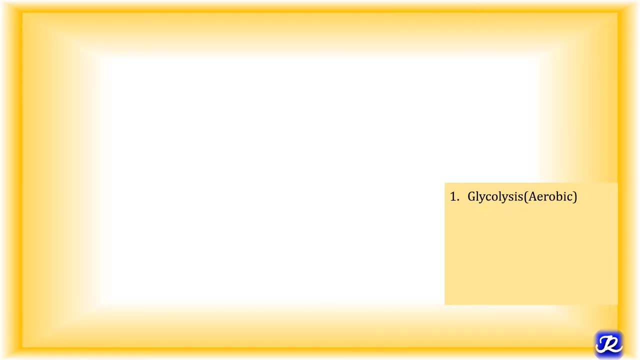 aerobic glycolysis. It is called as aerobic because it occurs in presence of oxygen. In this, glucose is converted into pyruvate through series of reactions. This pyruvate is then converted into acetyl-CoA, which further enters TCA cycle. The reducing equivalents are generated, which further gets oxidized through electron transport chain and, in presence of oxygen, ATP is generated and that's why it is aerobic glycolysis. But in some cells, which doesn't have mitochondria, because this formation of pyruvate to acetyl-CoA and further this oxidative phosphorylation occurs. in mitochondria. But what about the cells which don't have mitochondria? So in that condition, for example in red blood cells, this pyruvate gets converted into lactate, and this is called as anaerobic glycolysis. In addition to red blood cells, 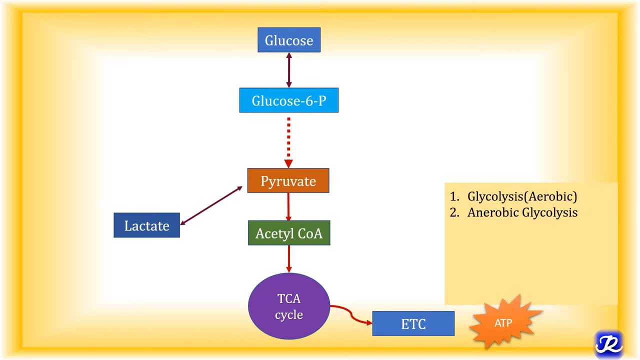 in the exercising muscle. also, whenever there is condition of inadequate oxygen or less oxygen, this anaerobic glycolysis occurs. So conversion of glucose to lactate through the pyruvate is called as anaerobic glycolysis. The third major pathway is glycogenesis, means synthesis of glycogen. 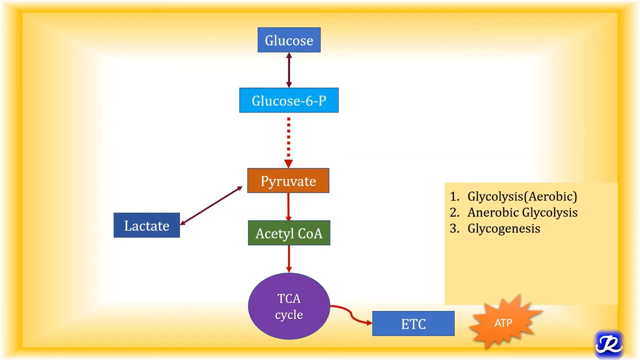 When this synthesis of glycogenesis occurs in the well-fed condition, whenever there is ample amount of glucose is present, the excess amount gets converted into glycogen, and this occurs both in liver and muscle. So the synthesis of glycogen from glucose is called as glycogenesis, which 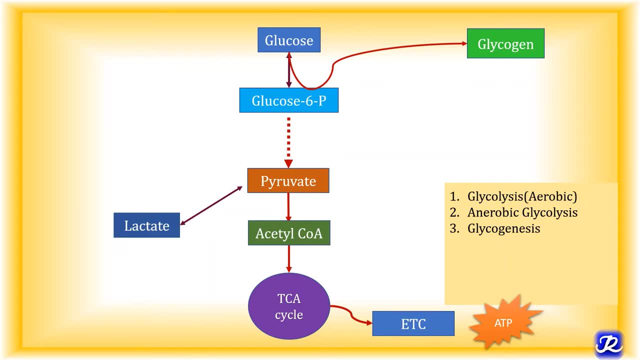 occurs in the well-fed condition under the influence of hormone insulin. The fourth pathway is glycogenolysis, which means breakdown of glycogen, That is, glycogen is broken down into glucose. So when this occurs in the condition of fasting and starvation, whenever there is no food intake, So in that condition, in the fasting state, 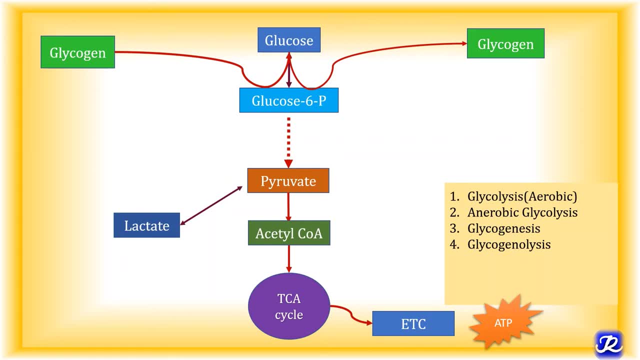 under the influence of hormone glucagon there is breakdown of glycogen occurs to form glucose and this process is called as glycogenolysis. Then the next process is glycogenesis. Gluco neo means new, genesis means synthesis. So formation of glucose, new glucose from the other. 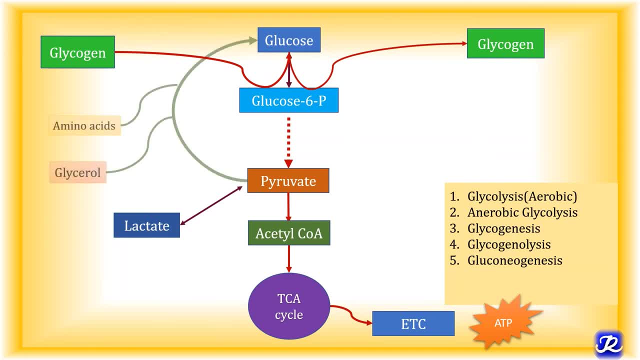 precursors which are non carbohydrate in nature, like pyruvate lactate, glycerol or some glucogenic amino acid. So if the synthesis of glucose occurs from non carbohydrate precursor, it is called as gluconeogenesis And again it occurs in the condition of fasting and starvation.